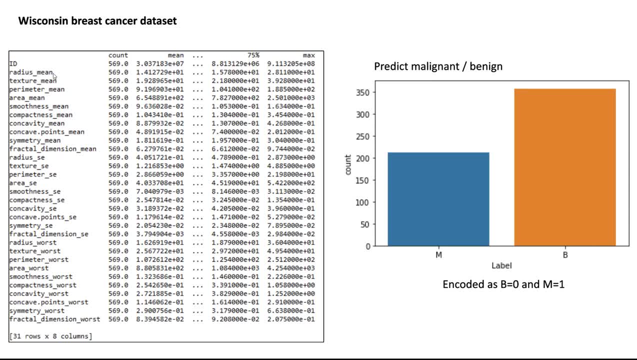 a bunch of attributes. As you can see, apparently, this is looking at, you know, some sort of a microscope image of this breast cancer, you know, probably a tumor, And it's looking at the radius texture, perimeter area and all of these parameters and predicting whether our goal is. 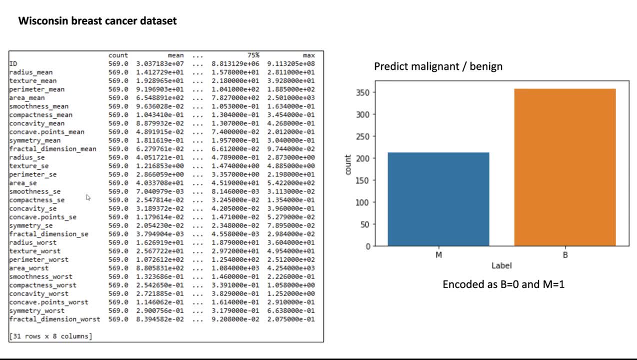 to predict whether it is malignant or benign And it's looking at the radius texture, perimeter, area and all of these parameters and predicting whether it is malignant or benign. So obviously it has the ground truth labels of malignant or benign. So let's fit this using our deep learning, You can 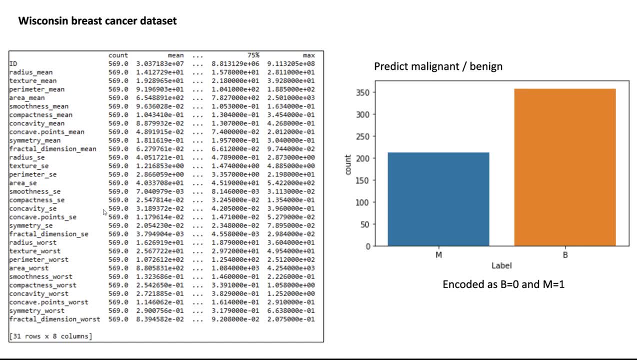 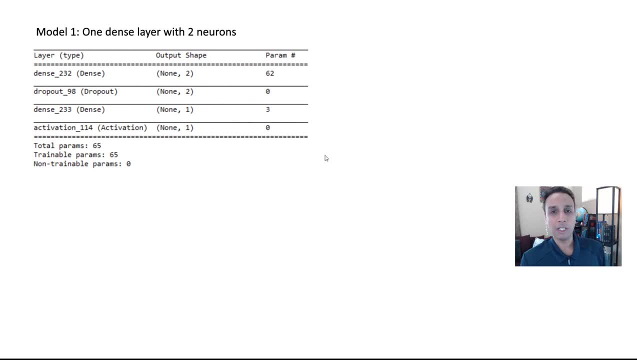 do this via the logistic regression if you want. okay, But let's look into deep learning for today. So this is the data set. Now let's actually build a few models to evaluate this data set. So I'm going to look at this from five different perspectives, right? So one is just a very simple. 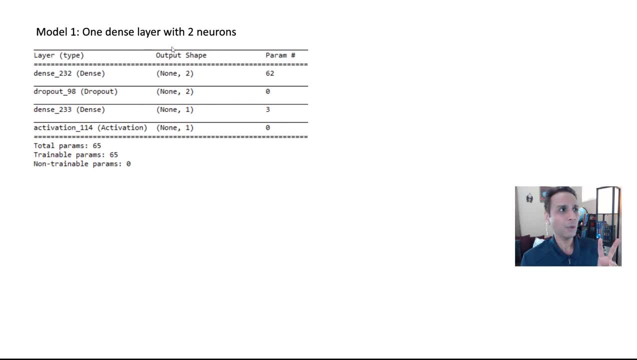 model: One dense layer with two neurons, that's it okay. So that's it: just two neurons, Maybe that's enough, And one dense layer with four neurons. In fact, I'll skip this part for today's video. You can do that. 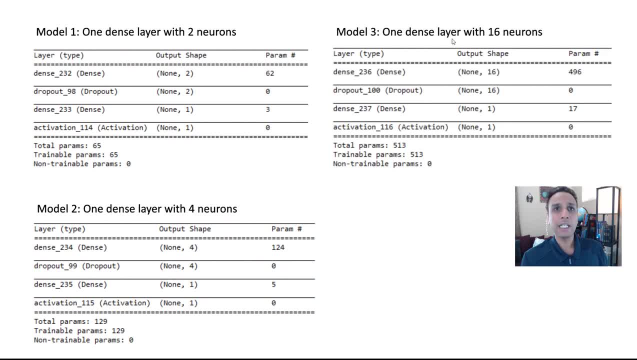 All you got to do is change this to four, right, And then one dense layer with 16 neurons. okay, Still one layer. So there are two ways you can actually design your deep learning model. One: increase the breadth right By going from two to four to 16,. 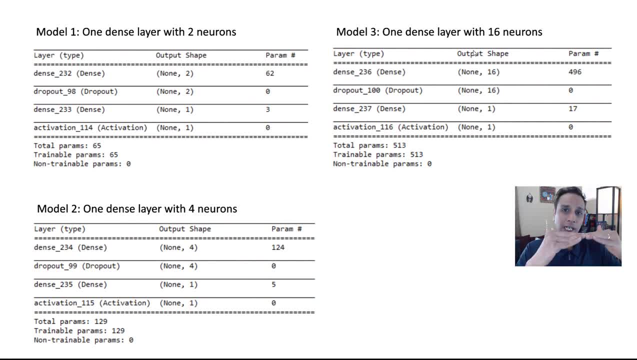 32 or 128. And two by going deeper. So instead of one dense layer you can do two, three, four, five, six different dense layers. Maybe I'll make a video on when to go deep and when to go breadth. 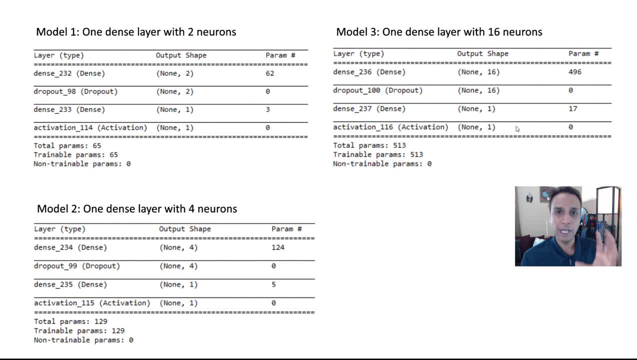 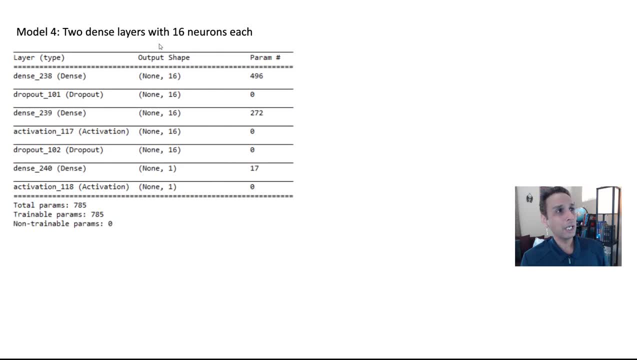 you know, in terms of breadth, when it comes to building your models, But for now, let's just focus on learning. you know the understanding, the loss curves, okay. In addition, I'll also look at two dense layers, each with 16 neurons. okay, Or nodes if you want. 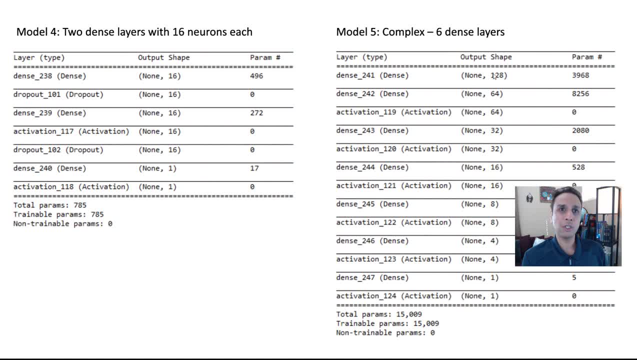 to call it, And then a bit more complex: six dense layers going from 128 to 64 to 32 to 16, okay, And you can extend this to your own problem if you want. you know that uses convolutional layers. Okay, now let's. 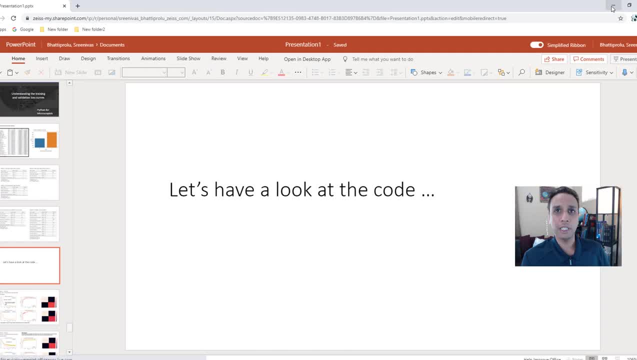 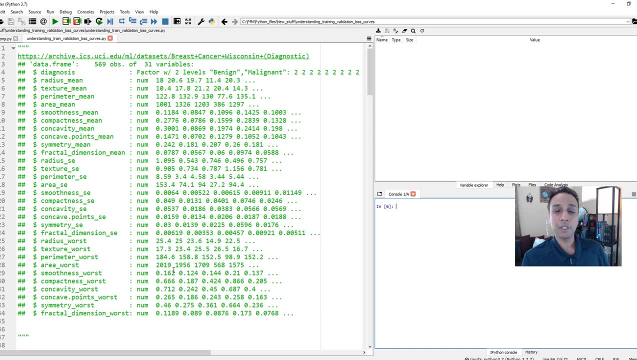 have a quick look at the code, So let me exit out of this presentation. We'll get back just to have a look at the results. But now let's look at our spider IDE. Again, I included the description As usual. I'll share the code on my GitHub page. Just look at githubcom. 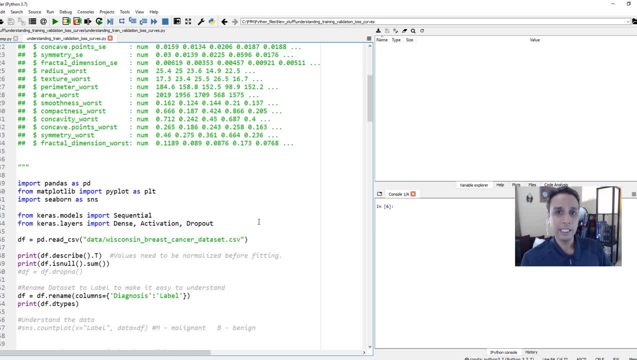 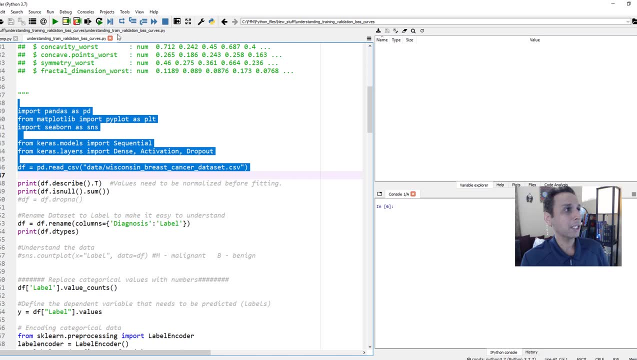 Or look at the description down here. you know as part of this YouTube video. Okay, so here again, I'm not going to explain the pandas part of it, I'm going to read the CSV right here. Okay, let me zoom on the. 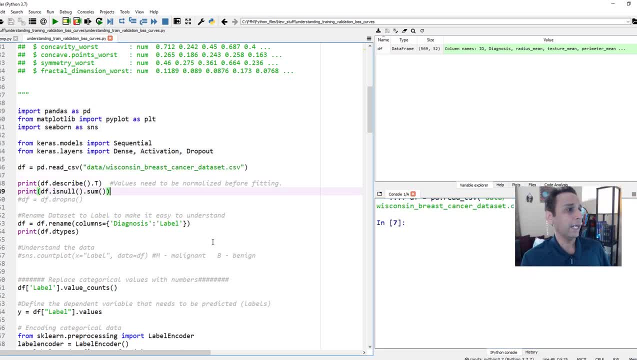 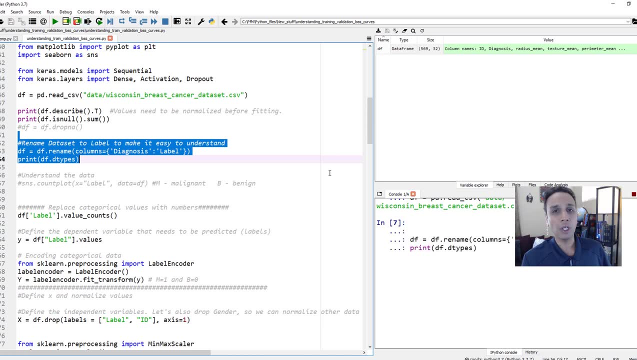 right-hand side so it's easy for you guys to see. Okay, so we don't need to do any of these. Let's go ahead and rename the diagnosis column as label, because one of the columns with the output you know, malignant or benign. 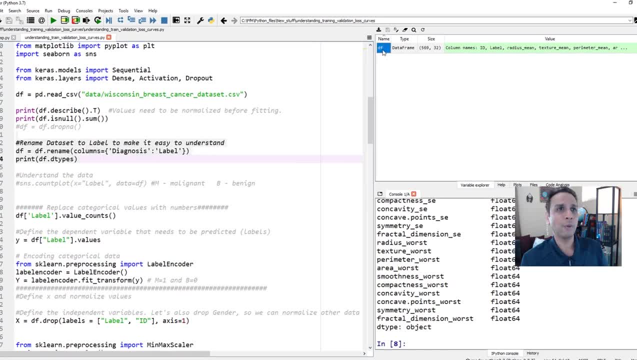 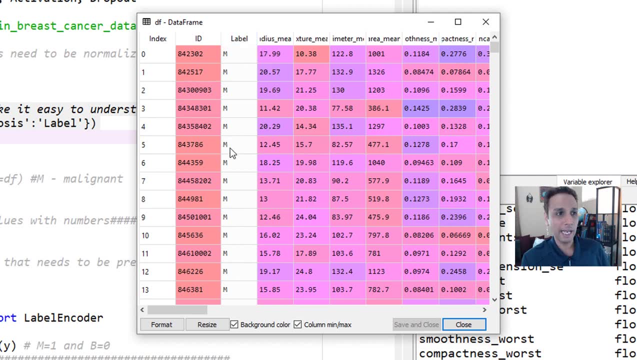 Is actually labeled, as is actually. let's have a quick look at the data frame. This column was labeled as diagnosis. I didn't like it. I changed the label. Now you can see it's M B. I think there's a lot more benign. 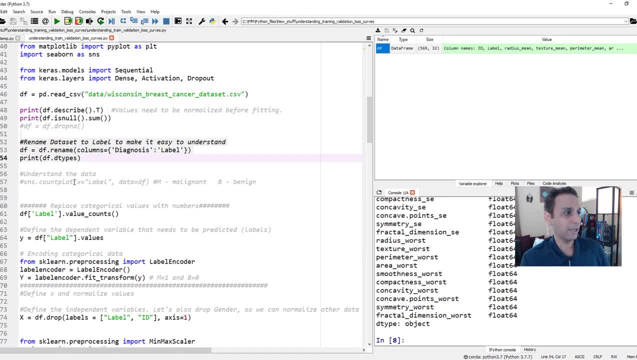 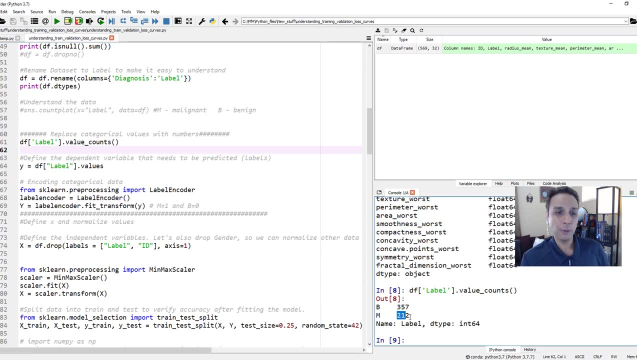 than malignant. But we can. we can get that information right away. So we just need to look at the value counts, And so we have 357 benign and 212 malignant. Okay, slightly imbalanced data set. Maybe you can actually watch my video. 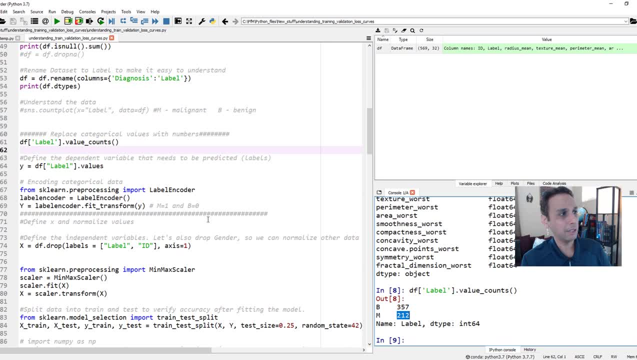 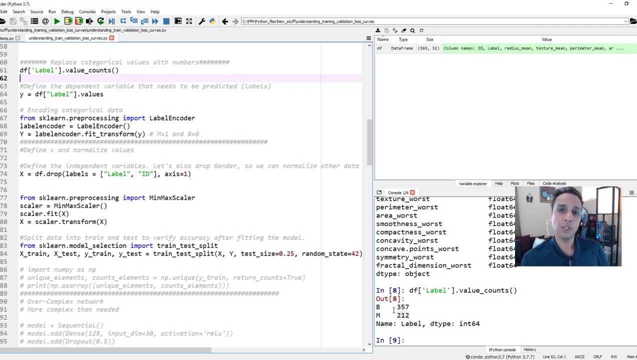 On how to balance data sets and try to balance it again. Let's keep focused for now. One thing you'll realize is: this is not much data. It is going to have an effect on how your loss curves look like, Because if you don't have enough, 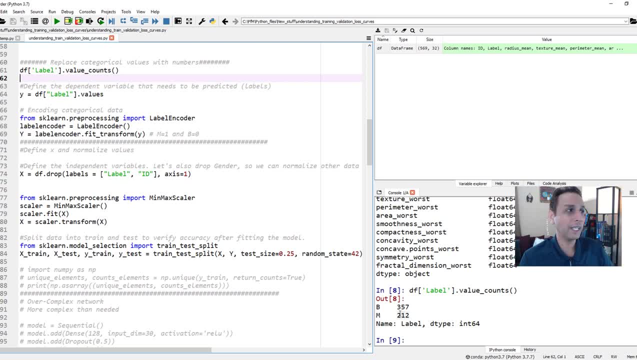 validation or enough training, then the curves may look different. Okay, so that's immediate lesson number one. And now let's actually encode the labels. instead of M and B, Let's encode them into one and zero. So that's what this is. Oh sorry. 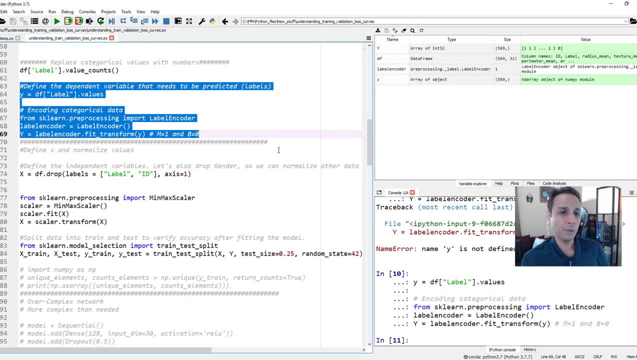 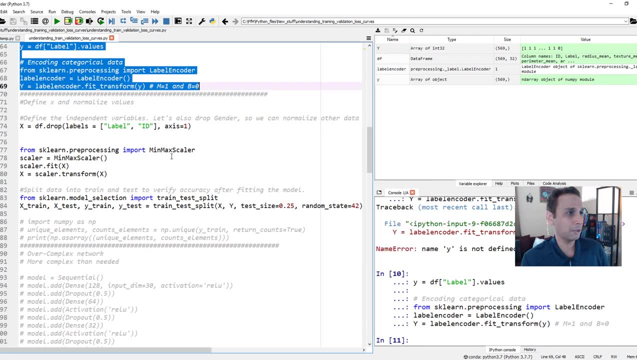 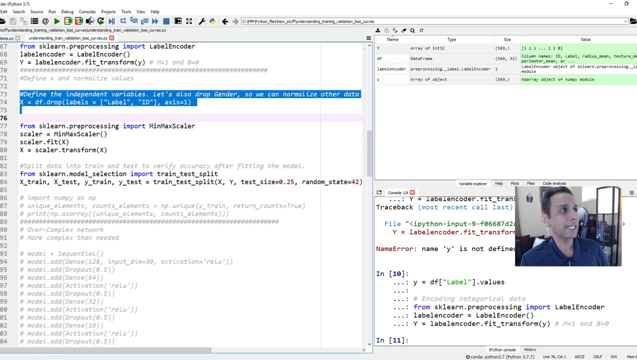 Let me that line and that's what this part of the code does. so if I open my Y right there, so it's now encoded as ones and zeros. okay, it's easy for us to work with, okay. and then now I'm defining my X. X is every column except for the column. 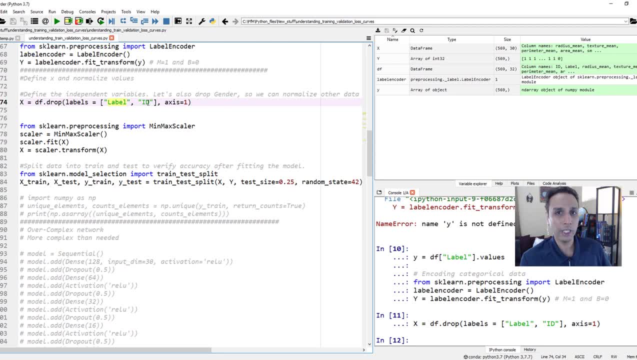 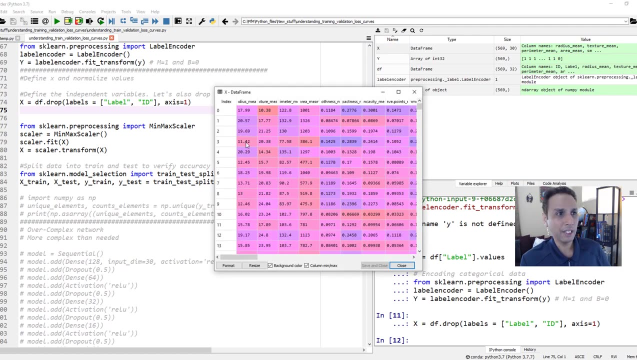 that's labeled, the label and ID. ID doesn't mean anything when it comes to fitting or predicting whether the tumor is malignant or benign. and my X values range too much. you know they differ in range. in fact. if I open this, you can see that the values go from 11, 77 386, 0.1. so it does make sense to scale them you. 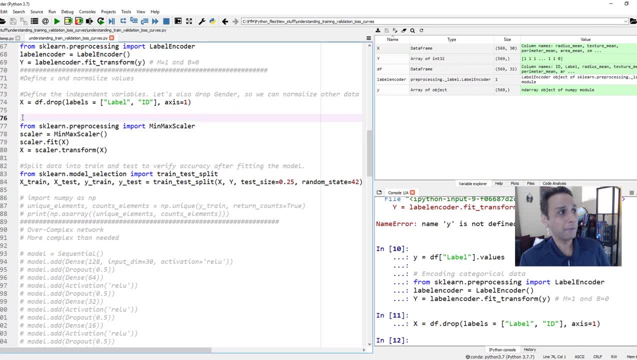 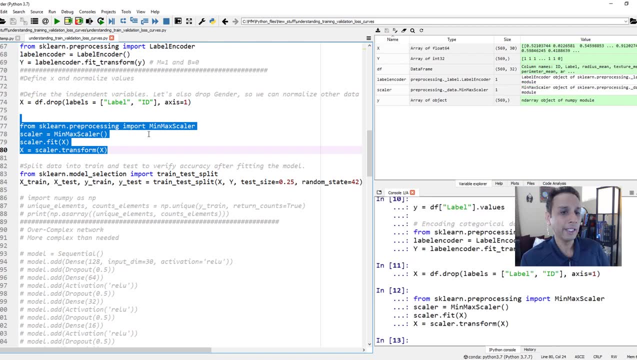 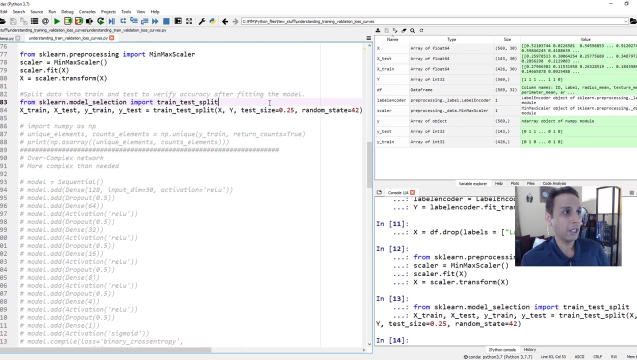 know accordingly. so our model is not. I mean again, this is another experiment that you can try to do. do not normalize and see how your loss curves actually look like okay, so let's scale it and, as usual, let's split the data. this is important. I'd like to spend a minute. 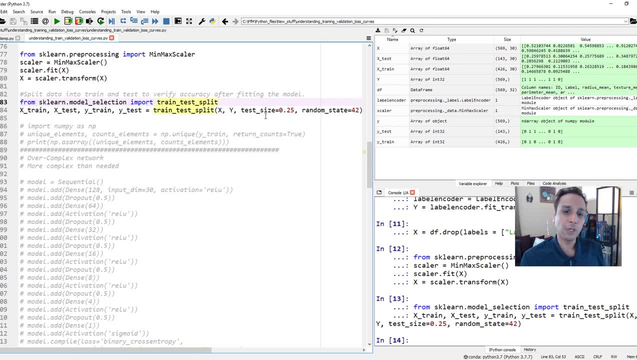 talking about this, but I'm not going to do that right now, so I'm just going to talking about this. every time we do deep learning, of course, or any type of data analysis in general, whether it is deep learning or not, you take your entire data set and you split them into training set and testing set, so you do. 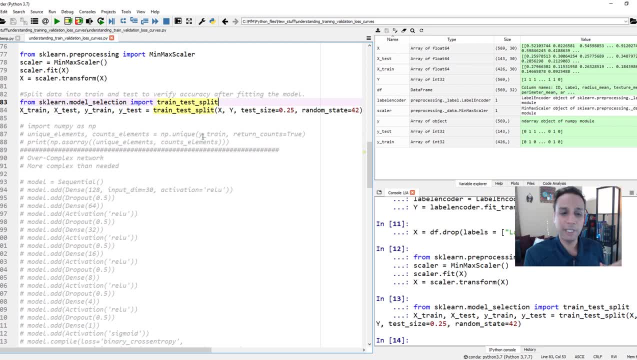 your model, building your model and everything using the training set, but then you validate that model using your test set. so the training never sees the test set. so this is: if you have additional data that you're holding out to test, that's even better. but this is a common way of doing things right and 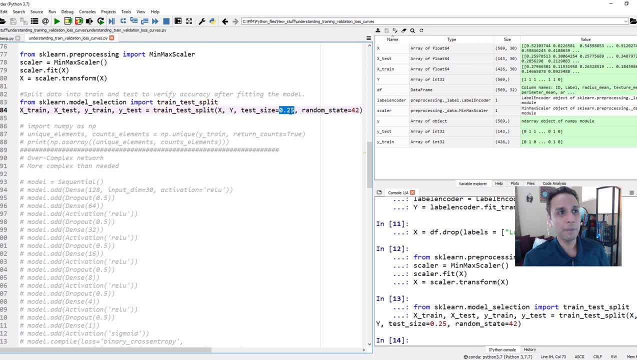 what is the best split size? this is another question that people often ask me- and the best split. I always start with either 80- 20 or 75- 25. if I don't have a lot of data, I'll probably do 75- 25. if I have a lot of data, then I'll. 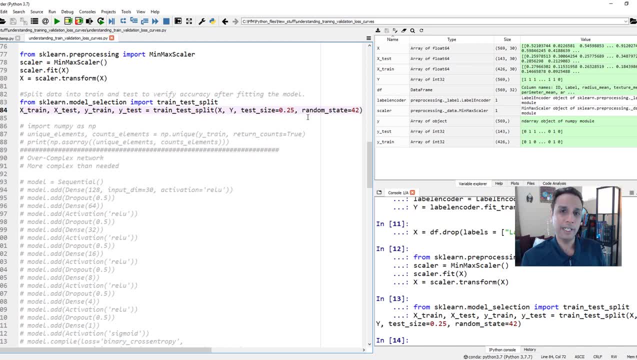 probably even go 90 percent for training, 10 percent for validation or testing. so there is no magic rule, but obviously you need to balance- you know the the amount of data between the training, because training requires a lot of their data and of course, you need enough diverse data as part of your testing set to do a 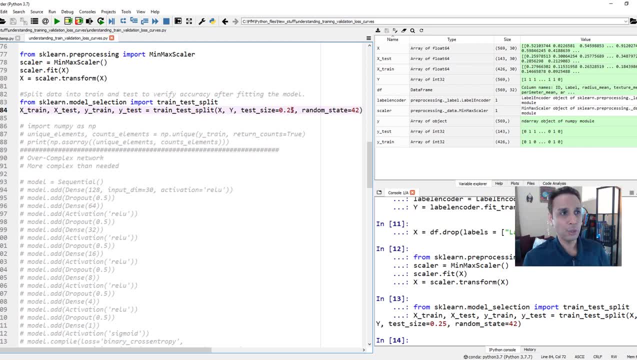 proper testing. so let's start with a test size of 0.25, which is 25% of the data assigned to test, and that's what I'm gonna do throughout my testing. now the random state, in case you don't use this. this can be very important when 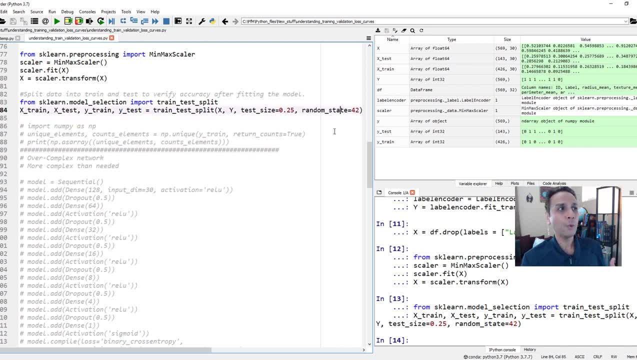 you are testing your models. so random state is how you want to split. because when you split your x and y values, you're doing this in a random way, right? I mean it randomly select certain certain you know data and then creates a train set and certain data creates a test set. so if you want the same train, 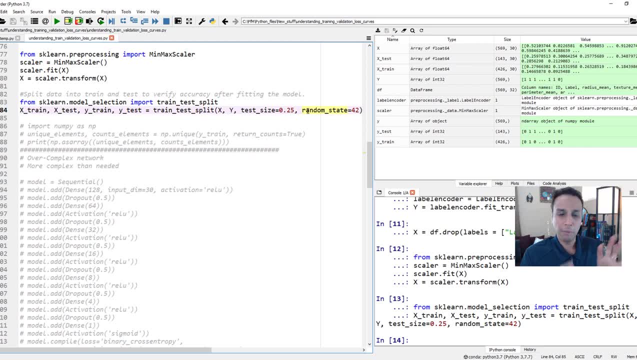 and test set all the time, because you're comparing the models. right then, keep this constant. now keep this constant, but change this value and then see how the model changes. because this split with a, with a seed of two, the split may look one way, but if I change my seed to something else, like 100. 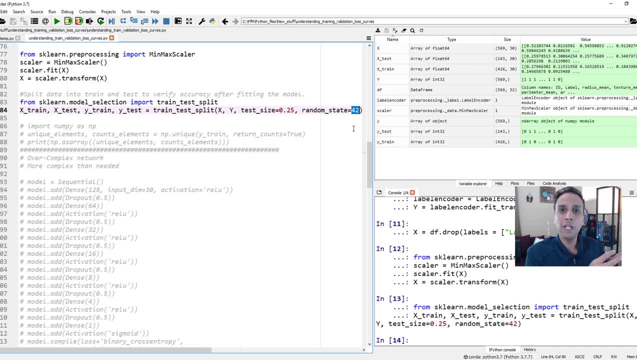 then the split may not be ideal, because maybe you have unrepresentative data in validation set compared to training set or vice versa. so it's very important for you to change this random state at least a few times to make sure that your model that you're building is working on the data, no matter how you split and dice. 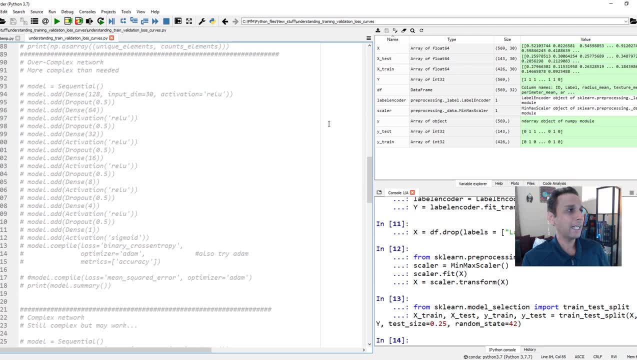 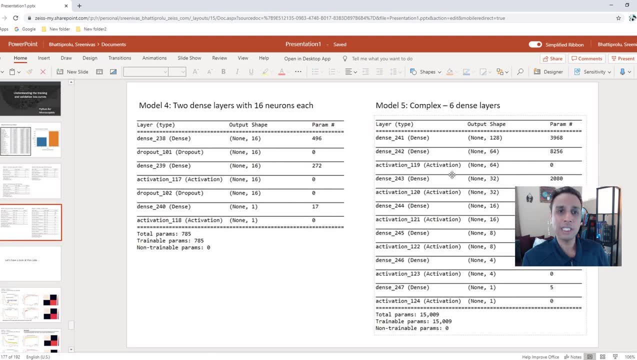 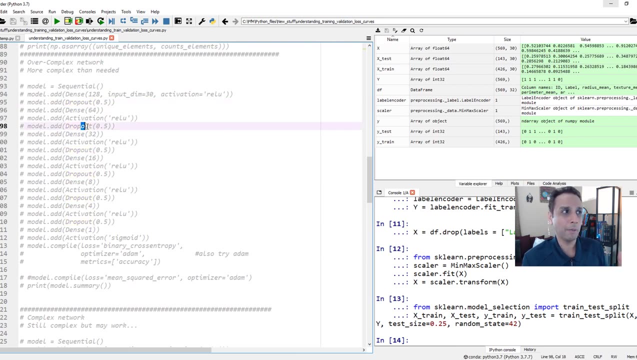 and slice it. okay, now let's move on. and then I defined a few model. this is the. this is the model I just showed you here, this one with six dense layers. okay, with six dense layers, I'm also adding dropout. we'll get to that in a minute. dropout is what is dropout before going from one. 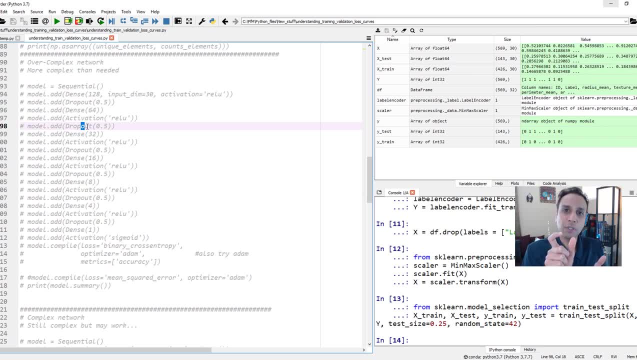 stage to the other, it drops out randomly certain percentage of data. and what percentage? if you put dropout, equals to 0.5. half of the data is dropped and then half is dropped and then half is dropped. why do you, why do you want to include dropout? 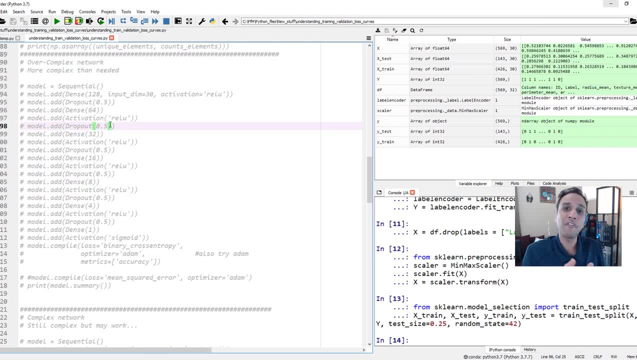 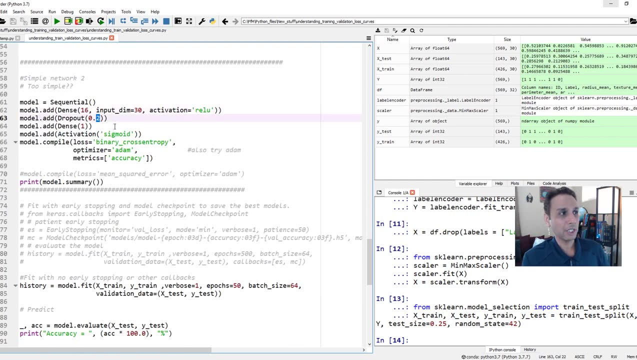 to make sure your model is not overfitting on the training data. so this way it's, it's a form of regularization. again, watch my video on dropout. okay, so I define my models here. so the only one I left here is the dense 16 with 20%. 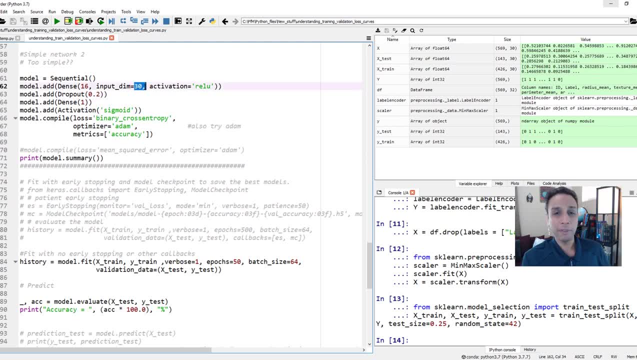 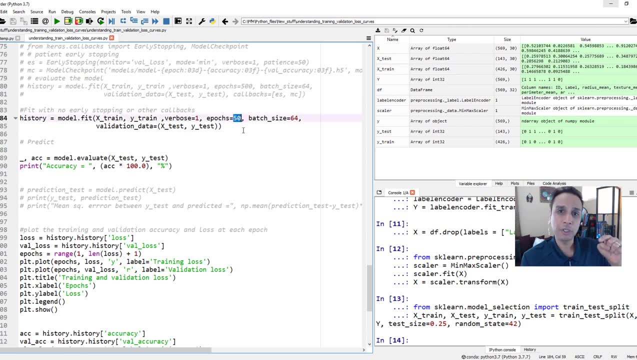 dropout okay, and we have 30 parameters that we need to model and everything else should be pretty straightforward and I'm gonna only do 50 epochs for the demonstration purpose. I have already on done 500 epochs under multiple situations conditions, so I'll show you the results in a minute, but I just want to show you the code. 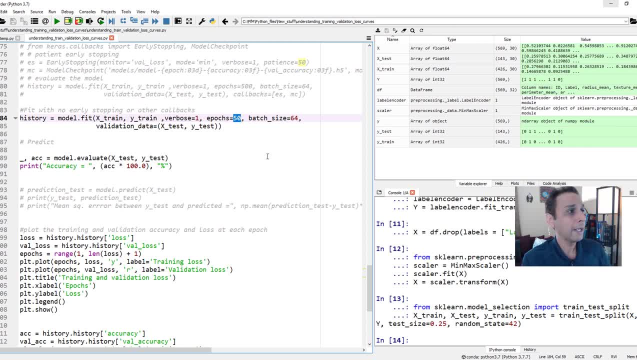 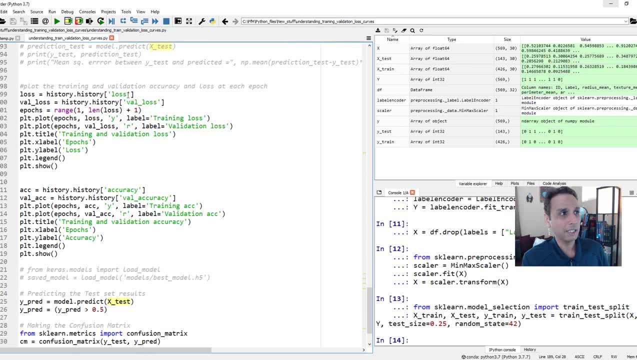 running so we can jump back into the presentation and continue it. ok, so after this, I'm going to tell you know, evaluate the model and I'm going to plot the. obviously this is why we are doing this exercise- right- the loss function for and the validation loss. okay, so both the training loss and validation. I'm also 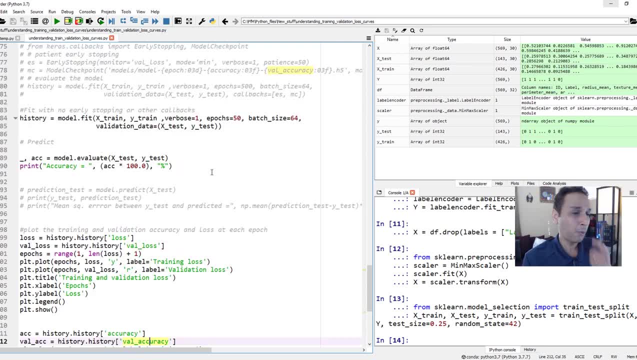 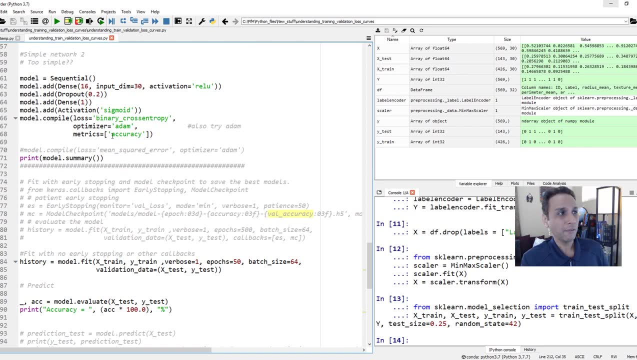 going to print accuracy and validation accuracy, then I am going to only do 10. now one thing that, in case you do not know if you are, As part of your model, if your matrix is accuracy Where you spell it out completely: ACC, you are a see why then down here you have to. from history dot history. 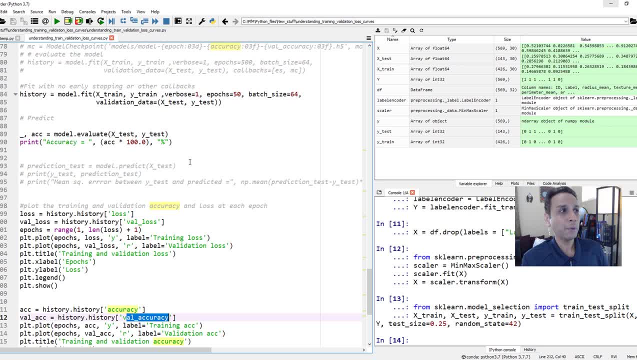 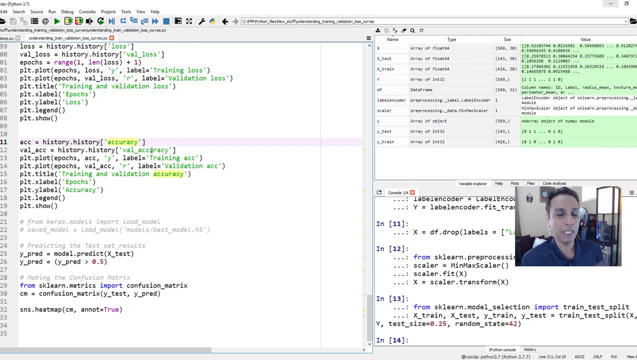 You have to do accuracy and well accuracy. if you put here ACC, then down here you have to do ACC and val ACC. Okay, this is a common mistake that most people do and I believe this changed in the in tensorflow to point something. But anyway, if it doesn't work out just by using ACC, you know why. okay, so this is the reason, okay. 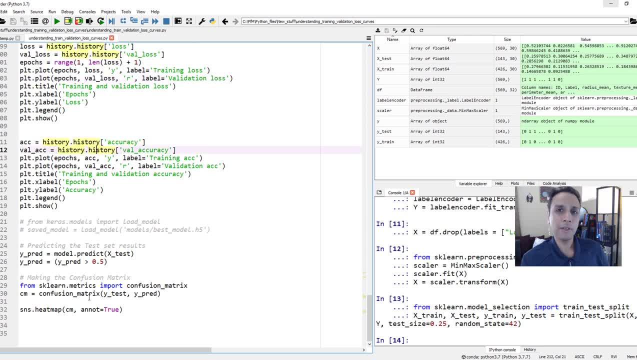 So we are going to plot these and I'm also going to plot confusion matrix to see how many false positives, false negatives and all That stuff. Okay, again, please watch my video on that topic if you don't know what I'm talking about. Okay, so, based on these conditions, let's go ahead and run this. 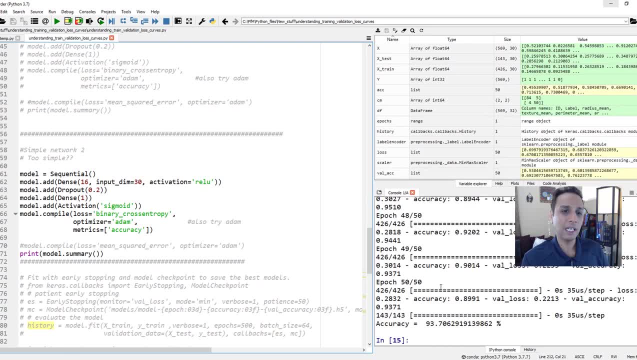 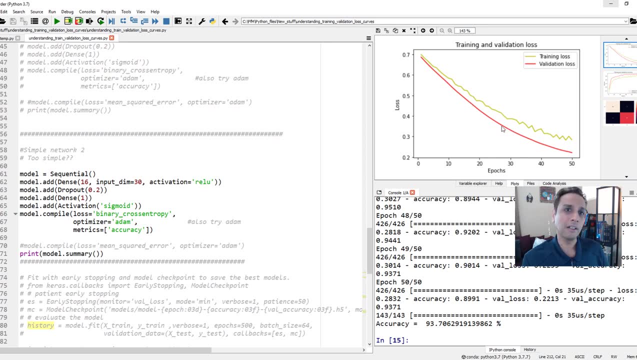 So it should Go for 50 epochs, which should be pretty fast, and let's look at the plots right there. Okay, so this is your validation loss and this is the training loss. and keep an eye here: The validation loss is below the training loss. Usually your training should be better, right? I mean, if the loss is lower, that means it's converging, you know. 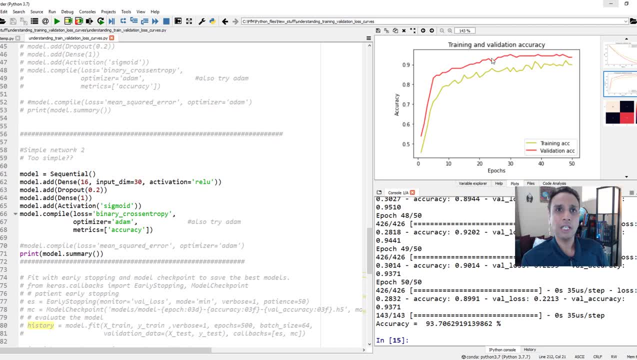 or if you want to look at the Accuracy, you see how- the red line, which is our validation- you're getting better accuracy and validation compared to training. Usually that's not the case. Okay, we'll jump to the presentation to understand why. yeah, and the confusion matrix is okay. 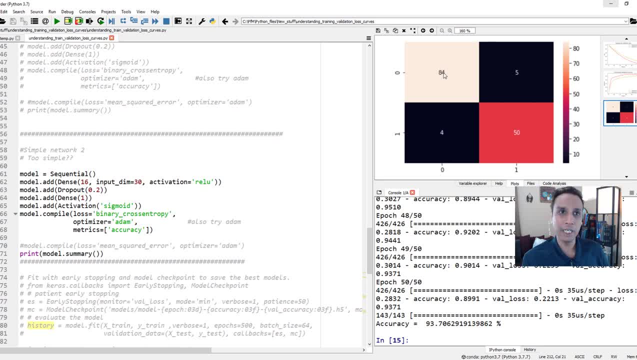 I have 84 benign correctly identified as benign but for got incorrectly identified as malignant, and 50 out of 55 malignants are correctly identified and five malignants are incorrectly identified as benign. Okay, so that's what confusion matrix is with this knowledge. Let me jump back to our presentation here and then. 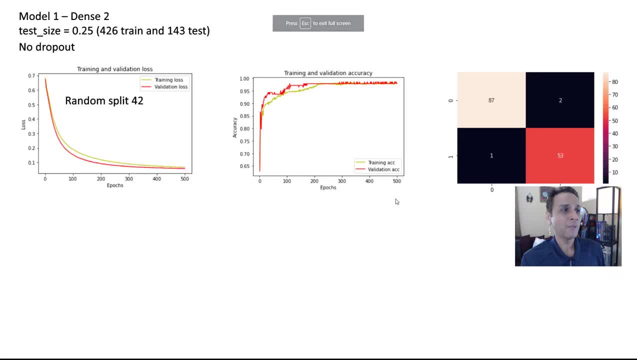 Have a quick look at some of the results that I got. Okay, starting with the very shallow, very small model, Dense, with only two. now I'll make another video in terms of what is the right model, how to approach, if I have time, But this may be too small of a model for this problem. Okay, complicated problems. 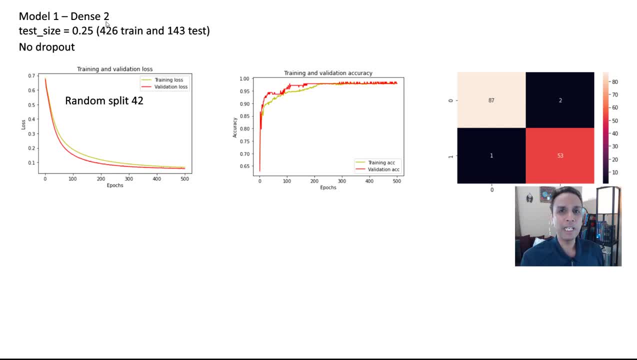 Especially with a lot of non-linearity, You probably need broader and deeper Simple problems. you can get away by just using very simple model, Okay. so if it's just a linear regression, then this would have actually worked right with two, three variables. But we have multiple variables, So, but still, this is not bad. This is actually pretty good, and I'm not using any dropout here. 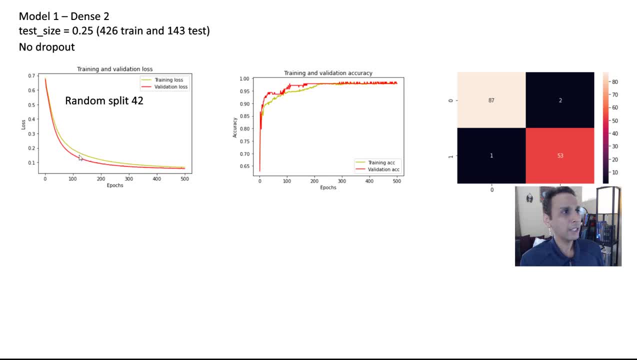 Okay, no dropouts in this case. So the training is going down and validation is also Is also going down. and the random split 42 just to show you that, okay, I'm split using a C 42 to randomly split, split my data and 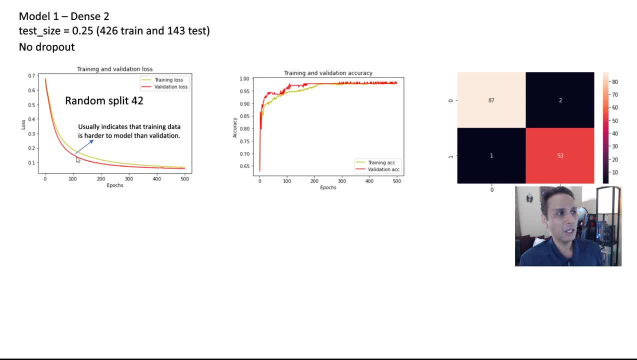 Now, if you look at why is this validation loss lower than the training loss, even though we're not using any dropout? That's usually indicates that the training data, the way we split it, The training data- is harder to model than the validation. and this, In other words, yes, it is harder to model, but this model may not be good enough to 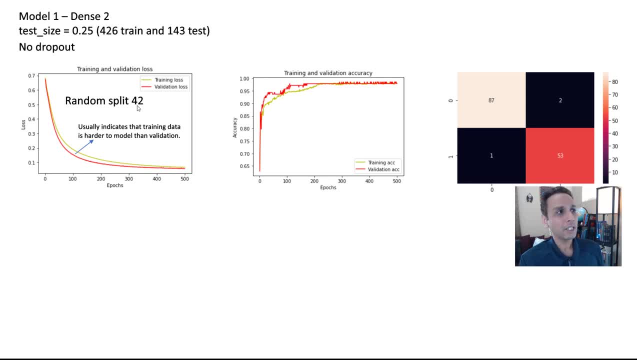 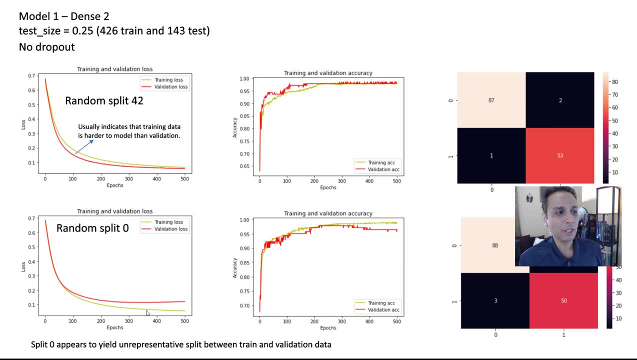 train, the training data. Okay, Now let's change the random split to zero and now you can see that there is a separation right here between The training and validation. you see how the training is lower right now with this split. Now it's seeing new data. I mean it's the same data, but for training it's seeing new data, for validation It's seeing new data, and. 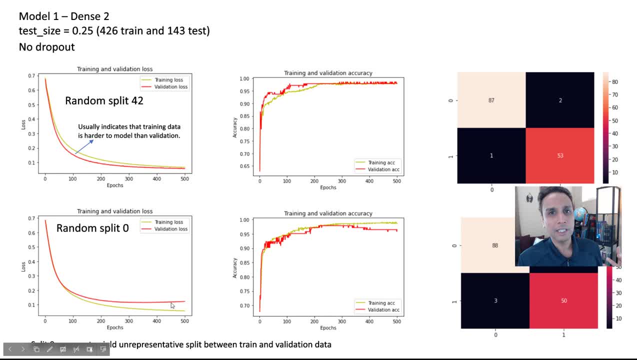 This appears to yield it's. it's about almost. we can say that this is Unrepresentative split between training and validation. It's not that bad if you want to read too much into it. The only thing I can say is the training and split our data are probably not. 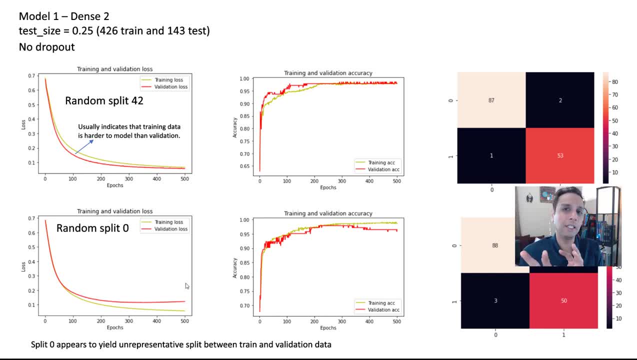 Representative enough, meaning you have slightly different behavior in the training versus the validation data set. Okay, I would still accept this. maybe at, You know, add some sort of our dropout to bring this validation a bit lower and then accept this. so let's do that. so let's actually add some dropper to see if it makes any difference, but not really, because this again I think, 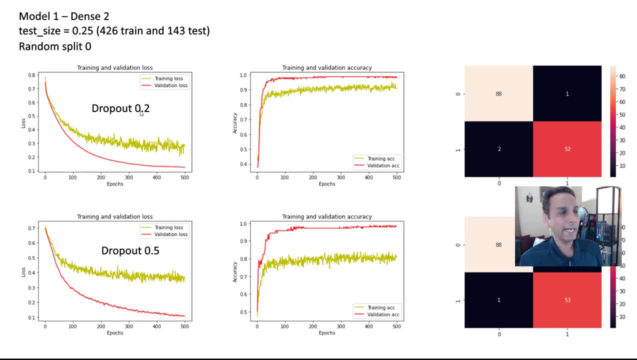 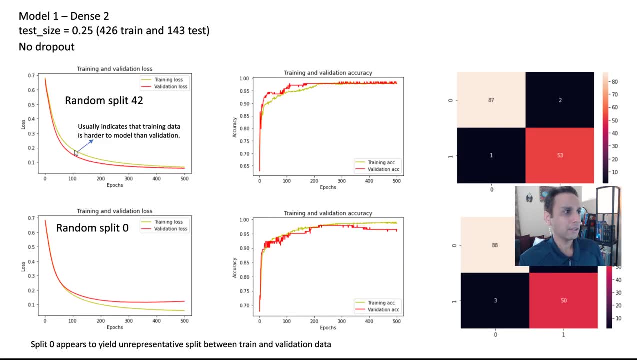 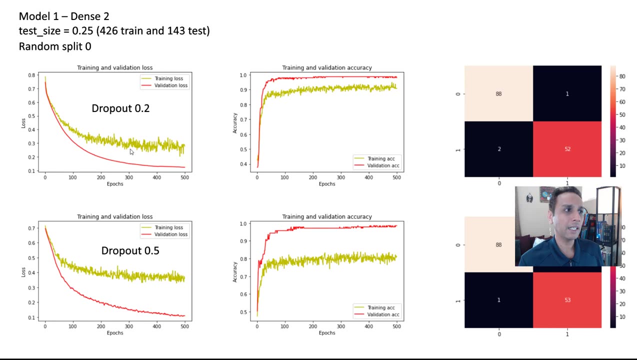 model is too simple. okay, you can see that by adding a 20% of dropout, my training loss is jumping up and down. you know, compared to my previous here, this is very smooth. now it's jumping up and down because we have limited data, so it's it's. it's working with limited data, so it's kind of jumping up and down, okay. 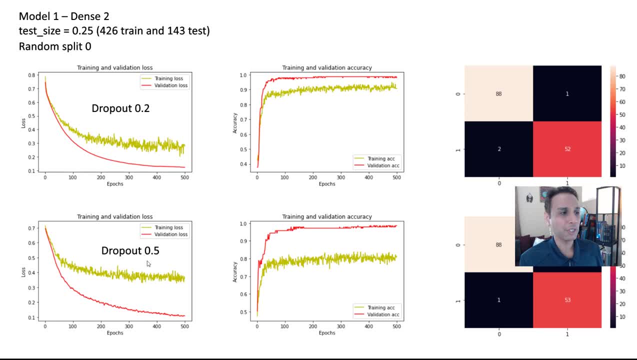 so the training and dropout with half 50% is even more, and the validation, so anyway, I'll. okay, I think I included this. I was thinking about whether I should spell it out or include. but now, why is this separation between these two right? I mean, why do we have our validation to be much lower than the? 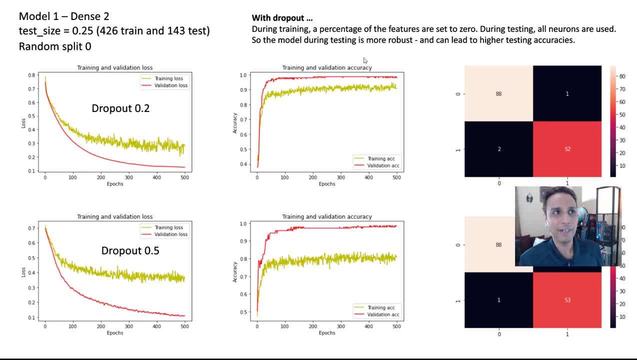 training- and I'm pretty sure you already read that here- because during the training process it uses dropout. it doesn't use dropout during the validation process, obviously. so during the training process, 20% of the features in this case, or of the, of the nodes you can say, or of the 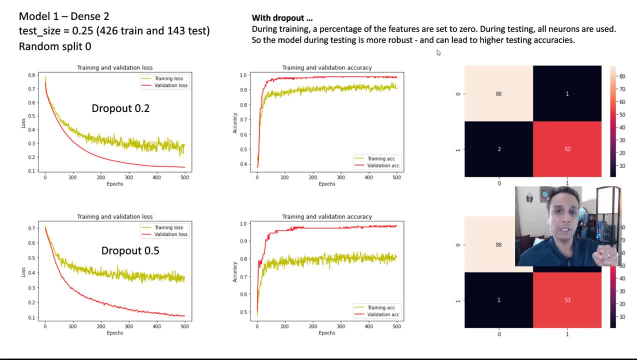 neurons are set to zero right because it's not using it. 20% are dropped. only 80 percent are used, but during the testing, all of the neurons are used. what does that mean? the model during testing is more robust than it is during training, so you lead higher. it leads to higher testing accuracies. that's why I 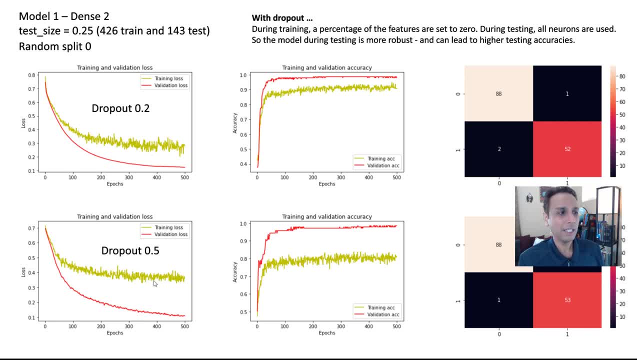 this indicates: okay, if you, if your dropout is aggressive, then you can see that the validation loss is lower. now the question is: is it acceptable to me? yes, it is acceptable if i see something like this, like dropout of 20 percent, where, yes, i understand why this is happening. so i would 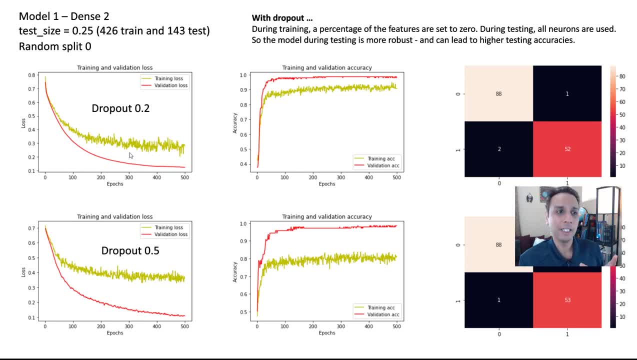 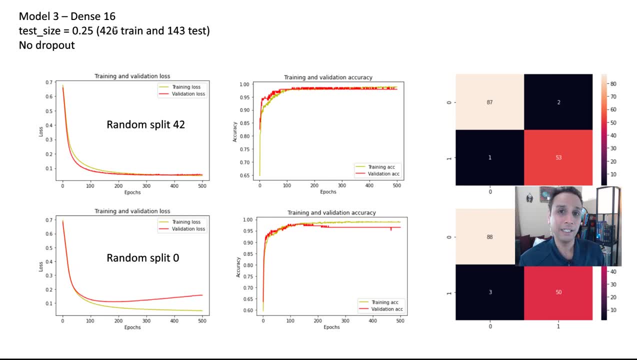 still test this on various uh splits of my data. okay, so this is lesson number one right now. now this model- the results you're seeing here- is with dense 16. remember previously we only had two neurons. now i have 16 neurons in the hidden layer. okay, so 16 neurons here, without 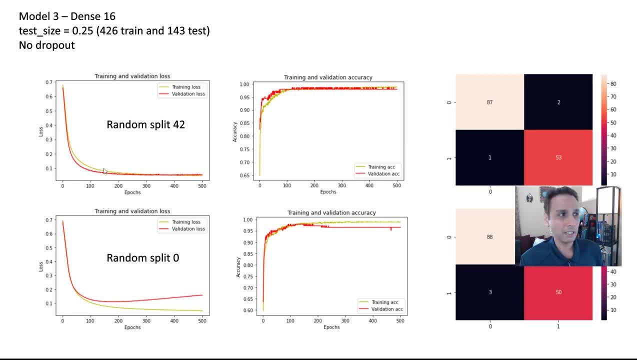 any dropout. that's an excellent curve, in my view. okay, this is. this is very good, because initially also they're correlated somewhat, not, but then eventually they're trying to come back together. this is great. now, that's for random split 42.. for random split: zero. whatever is happening. 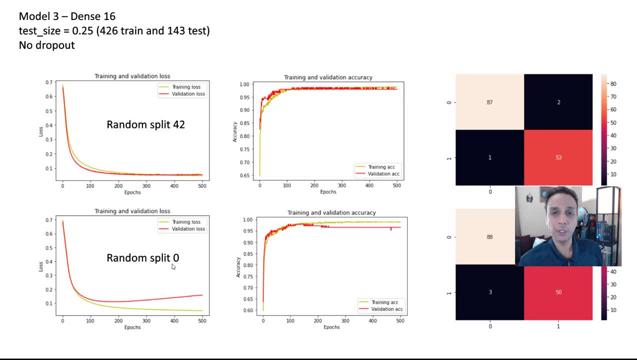 one of the opportunities is this: zero is very good for random split. 42.. random split is showing with random. if you you know, if you have time, if you're doing exactly the same thing, see why you know what's different with random split. what is the mean and average of all of these features? 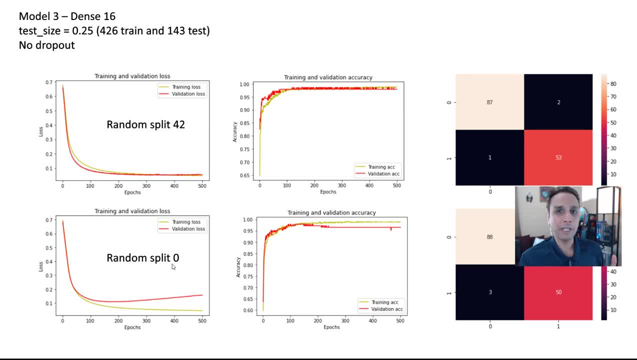 why is it different in zero versus 42? you know, again, people get masters and PhDs studying this type of stuff, but I'm just covering the surface of it. yeah, okay, so this is with random split zero. you have this type of behavior where your validation loss is, you know, going up and then. 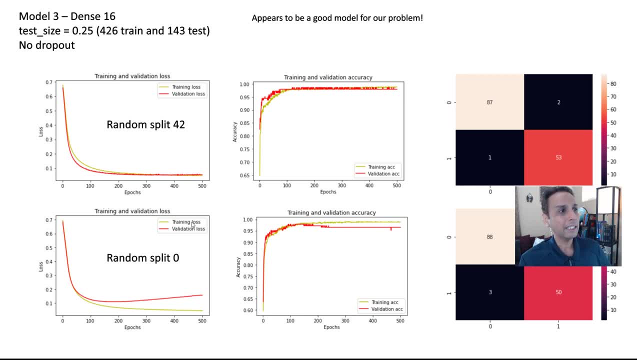 the training loss is going down right there now. I think this is a very good model for our problem, even though it's slightly diverging for random split zero. again, I need to investigate how this is now. can I, can I get make this any better by adding some dropout? I mean this different. I should 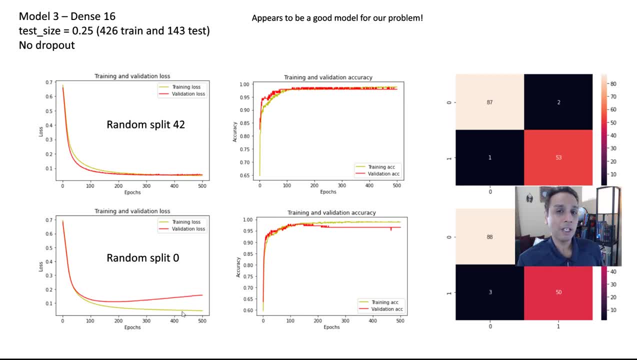 have mentioned this. this tells me that the day it, the model is working very well with the training data, but not as much on validation data for this split right. so that means our model is not different from the training data, but it's not as much on validation data for this split right. right. so that means our model is not different from the training data, but it's not as much on validation data for this split right. so that means our model is not different from the training data, but it's not as much on validation data for this split right. so that means our model is not. 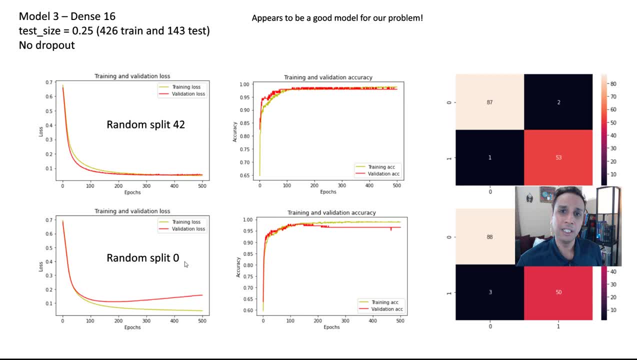 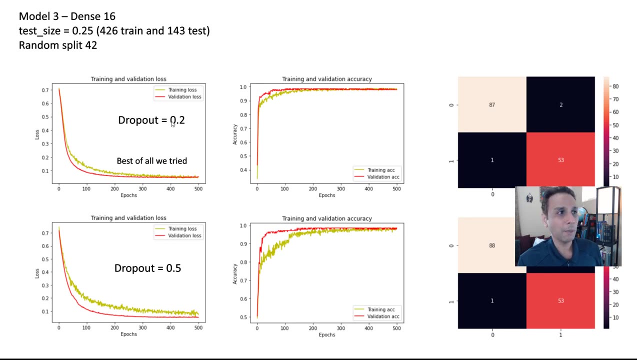 generalised enough to work on different types of data. so how can we generalize it? this is called regularization, and the way you do that is by adding dropout. okay, so this is the main advantage of dropout. so if we add the dropout, it gets much better actually. so, in fact, dropout of 0.2. 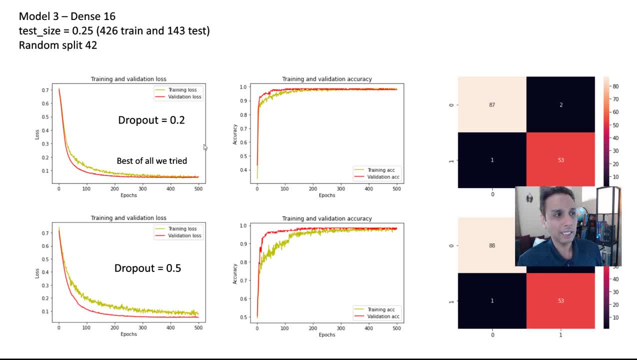 dropout of 0.5. it doesn't matter. usually in our dropout I try to stay 0.2 or maximum 0.3. if I have millions of data points, I can add 0.3, and if I have millions of data points, I can add. 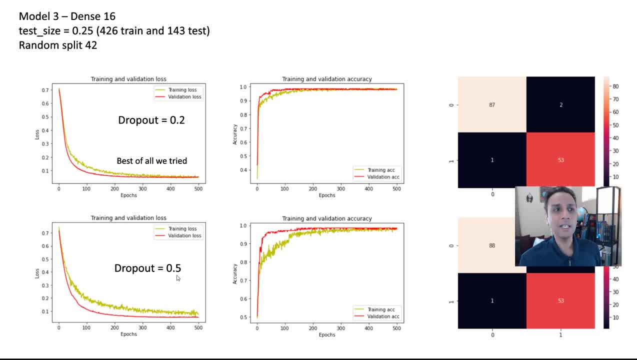 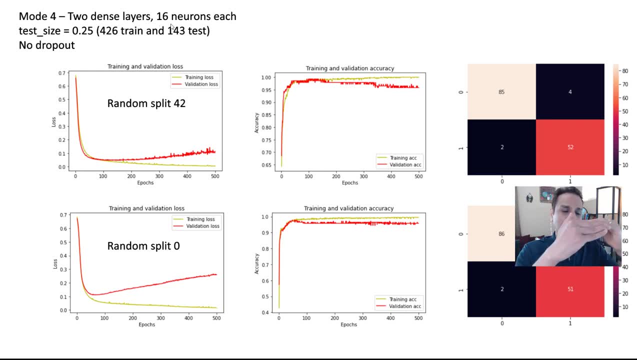 0.3, and if I have millions of data points, drop out of 0.5 is fine, but that's a luxury, okay, so now let's actually go to two dense layers of 16 neurons each. now we are increasing the depth. we increased to 16 and now we have 2 of these. okay, again, now you can see that it's actually. 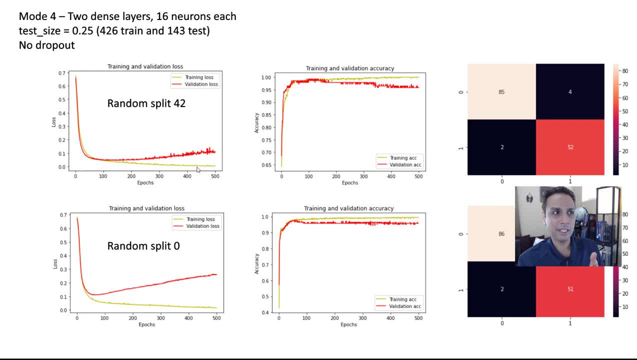 over fitting. you see how my training is doing excellent, but my validation is diverging. if I stop at 100 epoxy, maybe that's a good model. yeah, because after that the validation is such so I'm gonna get a Study doctor for a part that says the Validation, Quality of Validation is. 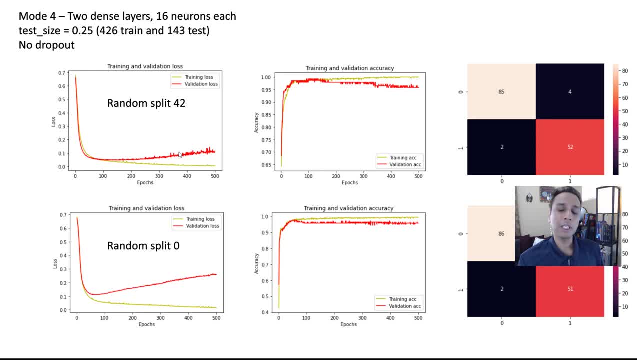 excellent. that is why I've created this model, because it's more a dissimilar symptom than loss is increasing. okay, if you put early stopping as part of your code, then this would have actually stopped at 100, because after that it's going up. okay, and this is even more horrible, right? I mean, to begin with a random split was. 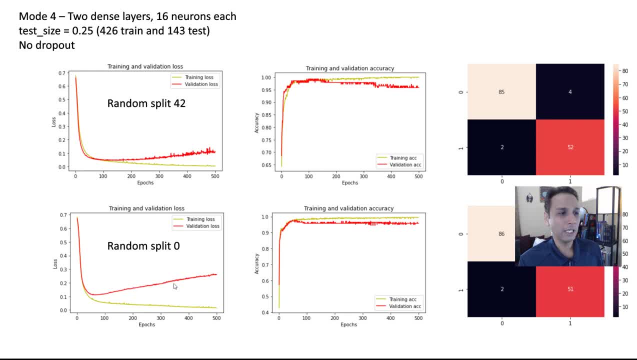 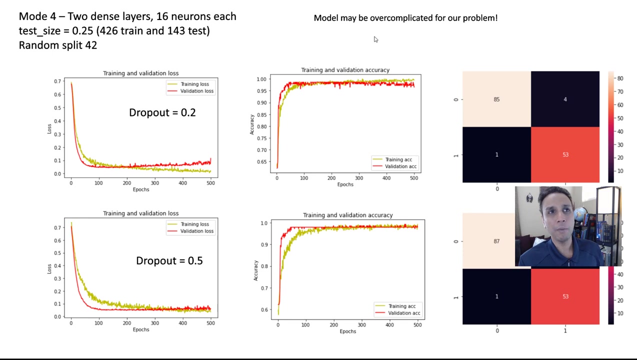 diverging for whatever reason, and it's going. the summary of this slide here is that with two dense layers, the model is a bit leaning towards overfitting, meaning it works great on the training data but it doesn't great on the test or other types of data. okay, now again, like I said here, maybe model may be. 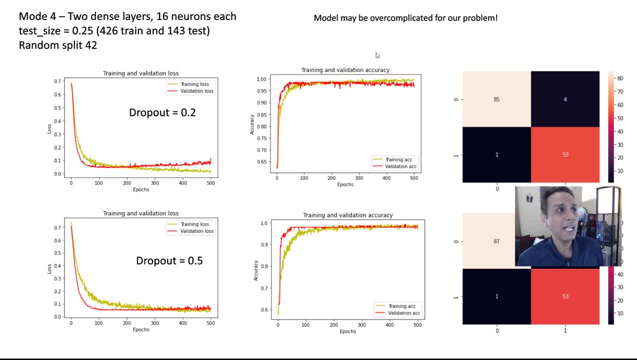 overcomplicated from the problem that we are trying to solve, and here I introduced dropout of 20% and 50%, so it seems to get a bit better. but I still think this model itself is a bit too complicated for this problem that we are. 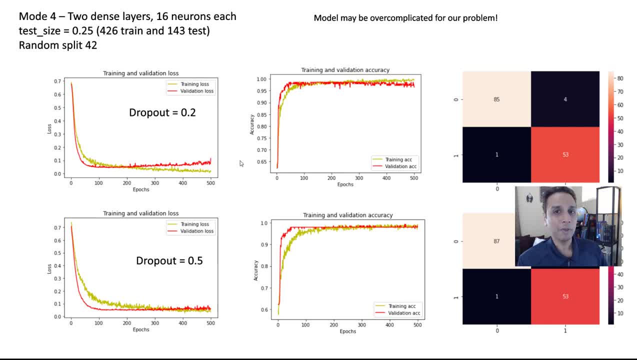 trying to solve now. let's make it even more complicated. remember the. the model itself is a bit too complicated for this problem that we are trying to solve now. let's make it even more complicated. remember the multiple six different layers, going from 128 to 64 to, and all that kind of. 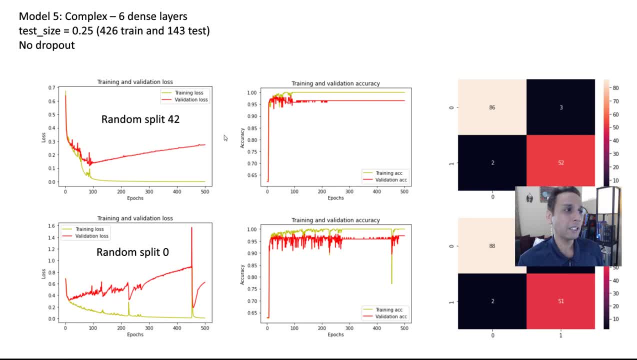 stuff, and this is the result of that. so if you see something of this sort when you're training, that should highlight that, hey, maybe the model is not right for the data that you're trying to work with. okay, maybe the problem is not as complicated, so you need to modify your model by probably decreasing the depth. 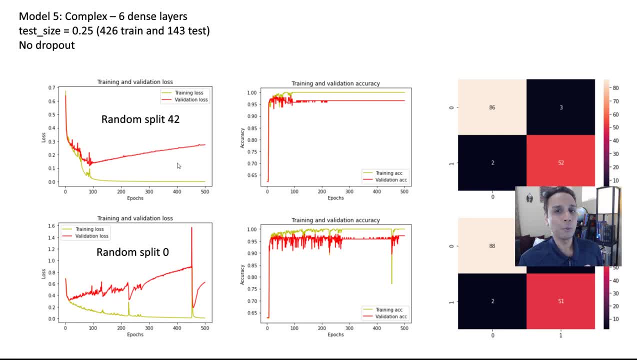 and also, you know the breadth, but I would start by decreasing the depth first. okay, so this is again a classic case of overfitting, where you can clearly see that the training is doing excellent, but the validation is doing horrible, and this is typically the case with very 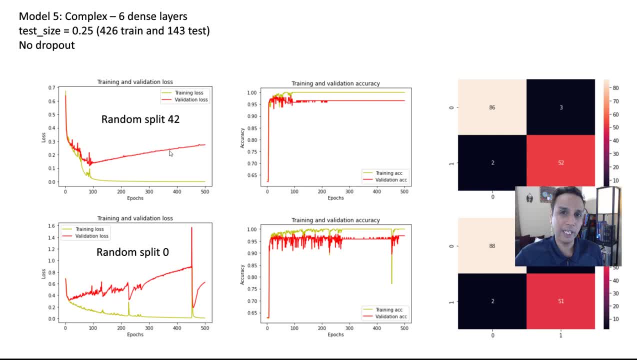 complicated architectures where you introduce a lot of hidden layers, because obviously you have too many weights and every weight is kind of represents something, and you may be even modeling the noise and all the other stuff that goes along with your data, which is not ideal, and with dropout also. I mean you can improve it slightly, but still you see how much. 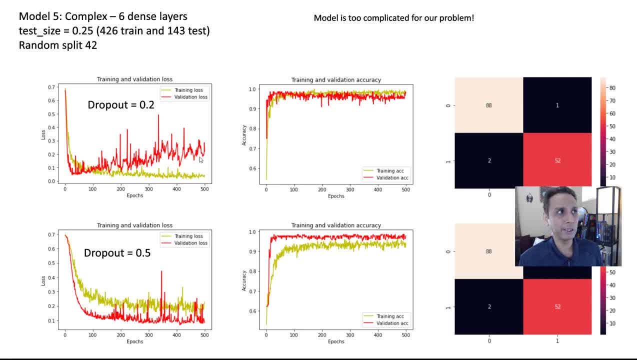 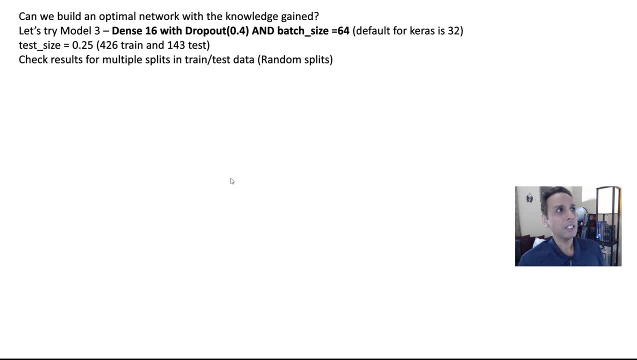 how much variation there is. so I wouldn't, I wouldn't go, you know, too deep for this type of problems. okay, now, with that knowledge, can we actually build? I apologize for a lot of text, but if you want you can read it out. but can we build an optimal network with this? so what did we learn here? well, dense 16 was. great, and now we're going to go ahead and we're going to go ahead and we're going to build an optimal network with this. so what did we learn here? well, dense 16 was great, and now we're going to go ahead and we're going to. 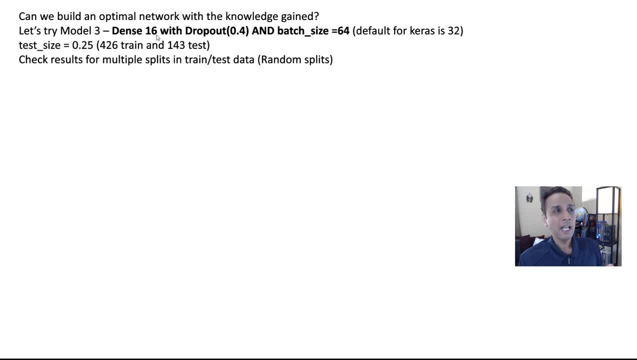 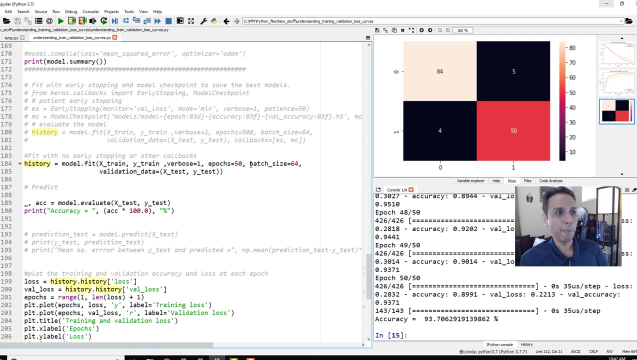 it gave us decent results. it had a dropout of 0.2, so let's try dropout of 0.4 and let's also change the batch size. this is very important. I haven't done that experiment, but if you actually go down, what I mean is when you do this. 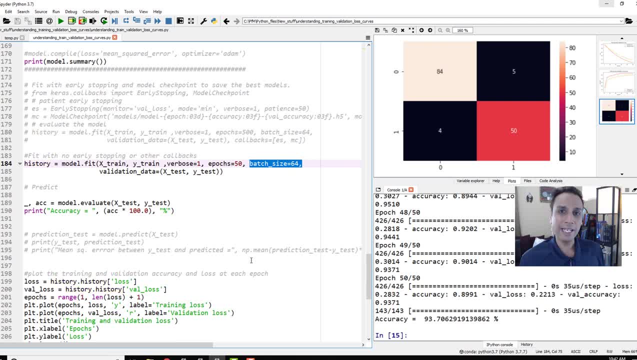 batch size. if you don't mention anything, the default batch size that Keras uses is 32. you probably need more data points per epoch yep per iteration. sorry, you probably need more data points per iteration to fit the model. so you can try batch size 64 or 128 and see how that affects your. 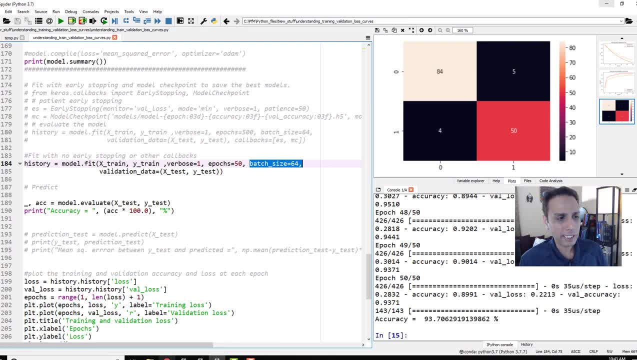 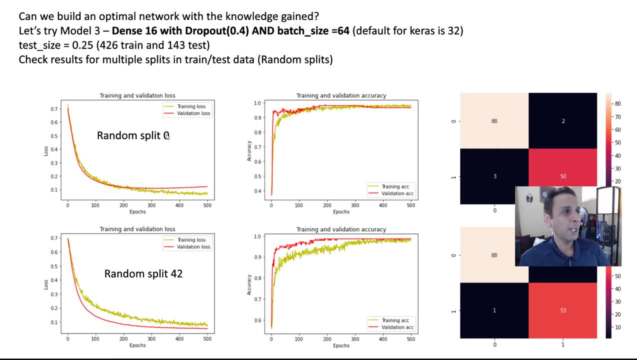 training and validation loss curves. okay, so let's get back. so that's the batch size I'm talking about. so let's see if we can actually get a better model. and I'm doing multiple split, so with random split zero. this is what I got got. remember, our seed zero was the troublesome seed that's giving us some weird split in the 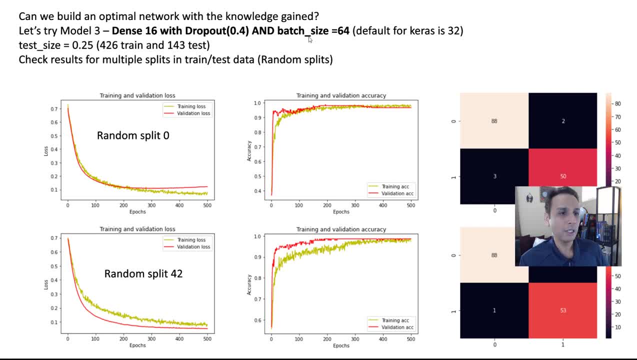 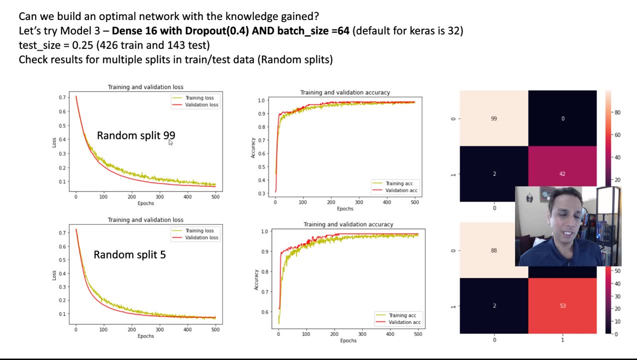 data, but with a random split of 42 with under. with these parameters i'm getting a very decent curve. maybe i can increase the training for another 100 or 200 epochs to get a better convergence between training and validation. and random split. 99. i just did a whole bunch of these. 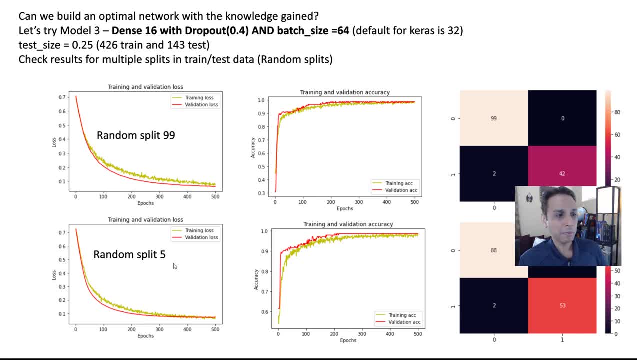 i'm just showing four or five, uh, also converging random split of five is also converging at about 500 epochs in this example. i also did a whole bunch of these and they all seem to give me a decent. except for zero, everything was acceptable. so i thought, okay, this is a great approach, this. 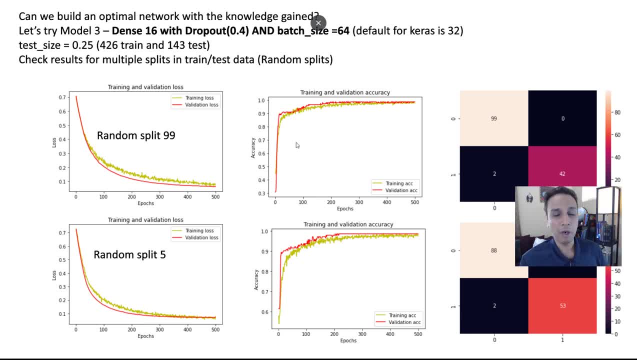 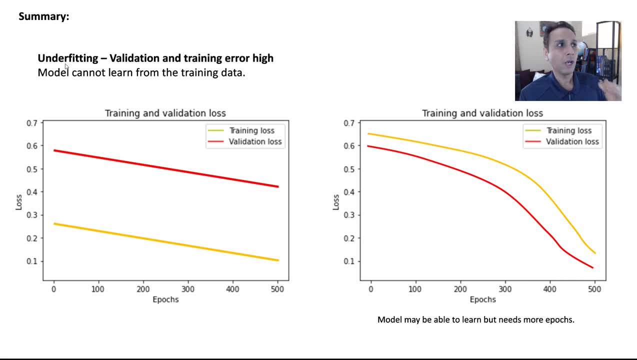 is how, if you're starting from scratch, this is how you can actually build your model. so let me summarize the learnings here. okay, the there are, uh, to introduce a few terms, there is something called underfitting. underfitting means you have validation and training. error is very high and it can appear in multiple forms, but typically, if you 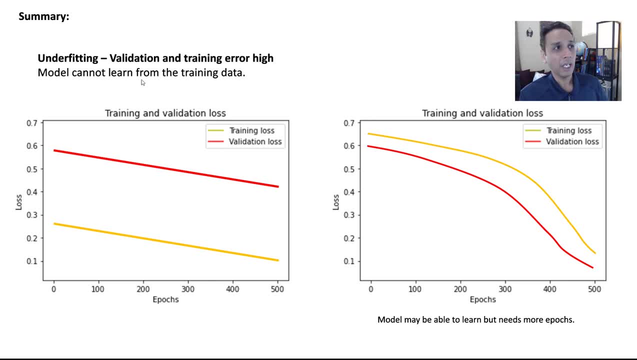 see something like this: the error is pretty high. that means model cannot learn from the training data. you need more training data or the training data is too complicated for this model to learn from. so increase the depth, increase the breadth, you know, change the architecture. so that's uh. 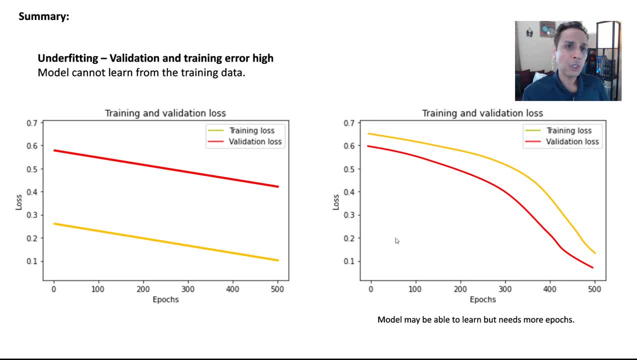 uh, you know, to address the underfitting, it can also show up like this: and: uh, this is a good, relatively good, sign. still, i would try to change the model a little bit to fit the problem, but in this case there is some hope. yeah, model may be able to learn, but it needs a lot. 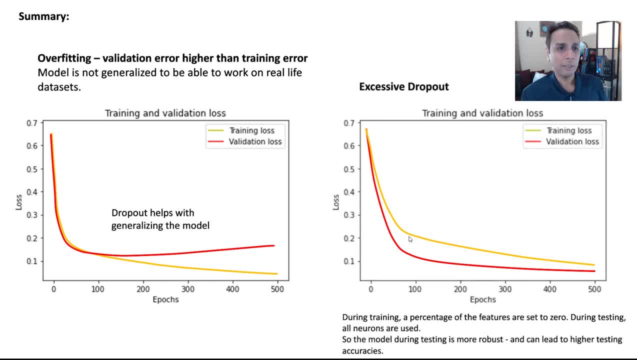 more epochs. now, overfitting: we already talked about overfitting. sorry about the animation there. the overfitting is, uh, the validation error is higher than the training error. yeah, so we already saw this in a couple of examples. you see, the training error is lower than the validation error. 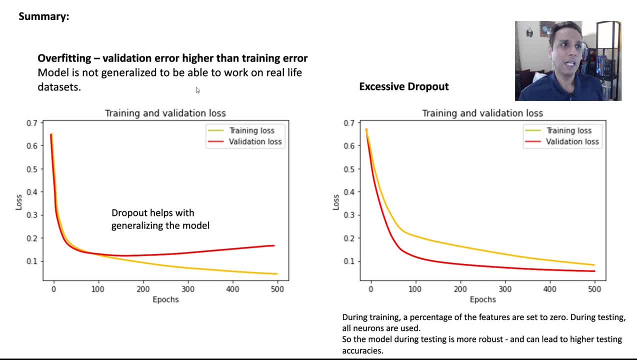 that means the training error is lower than the validation error. so the training error is lower than the training error. that means the model is not generalized enough. uh, to work on real life data sets. okay, and, as i mentioned here, dropout helps with generalizing the model. so, uh, now. but 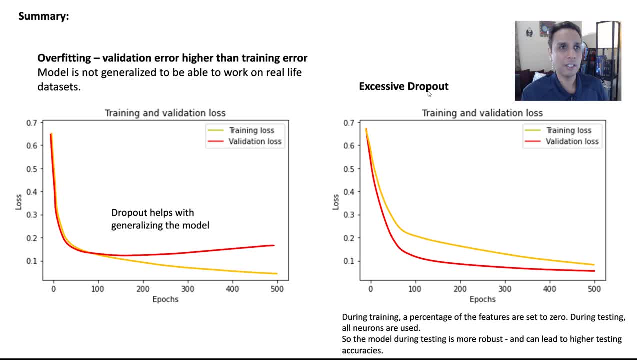 the problem is, if you do excessive dropout- yeah, we already saw this again- then your validation accuracy or the validation loss is much lower. validation accuracy is much higher than the training accuracy right, which is acceptable in my view because i already gave you the reason, right. i mean because, uh, we know that, okay, during training it's dropping out, so not much. 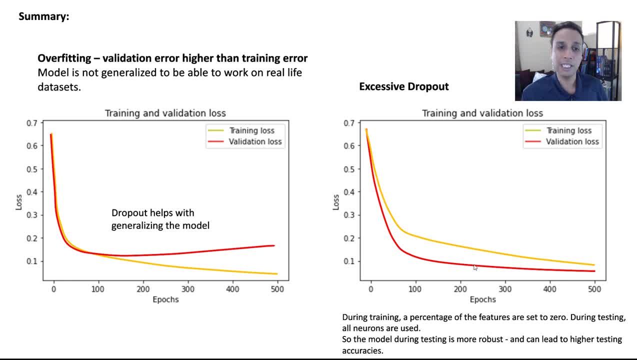 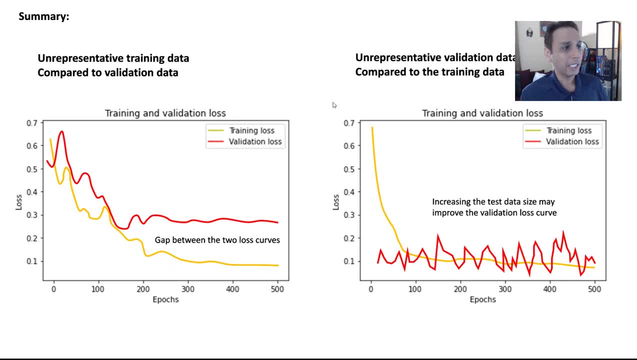 data is available, but the model is much more robust during the testing phase. as long as you understand what's going on, that's the key point here. okay, finally, let's finish this off by looking at a couple more examples. so one here is unrepresentative training data compared to 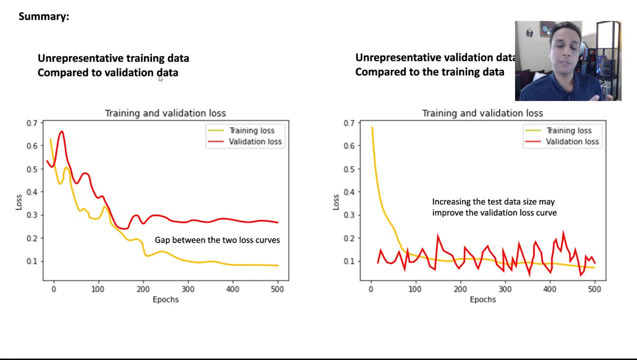 validation. i think that's the case. when we looked at, uh, the split at zero, uh, you know, with our seed equals to zero, which is okay, you're not going to be able to do that. you're not going to be able to do that, you're getting a split. but then the validation, the statistics that, uh, you know of. 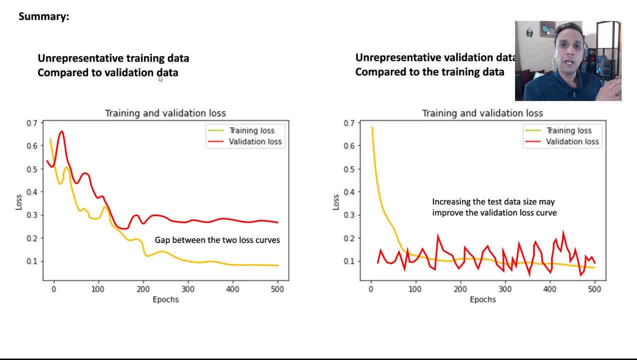 your data in the validation set are different, i should say, compared to the training data. so when that happens, then of course the model will be training, but then there exists this gap between the model and, uh, you know the training and the validation part. so shuffle it and then try this. 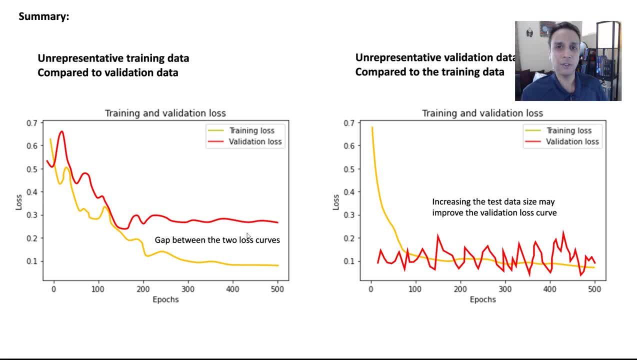 one more time. okay, or try to artificially enhance your data or collect more data. of course, that's always the answer, but find a few tricks to actually eliminate this. now. if your validation data is unrepresentative- meaning you got like excellent training data, but then the validation data- you only have 10 data points. if you don't have enough data points, 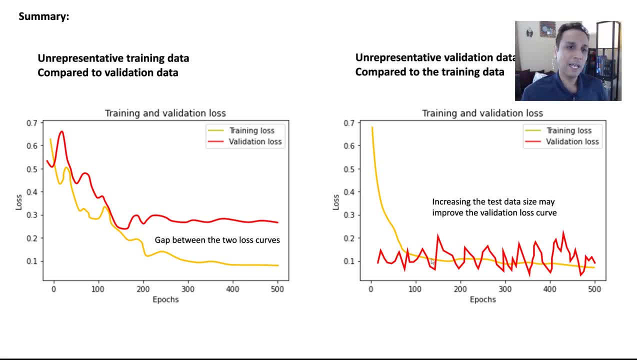 that represent the training model. then you may just have results that just jump up and down. yeah, this can be the. the accuracy curve also looks very similar to the loss curve in this case. okay now, uh, so after all that, how does that work? so let's look at the data set. so let's look at the. 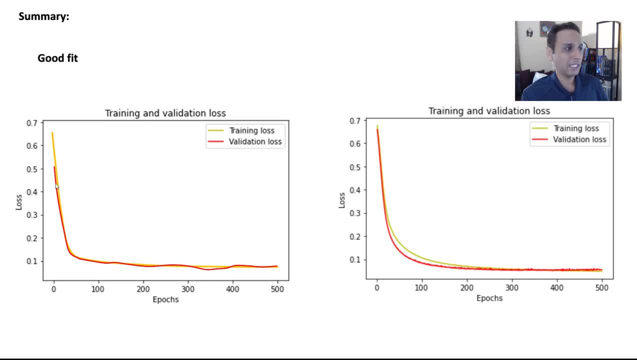 good look. uh, you know good fits actually look like and, as you can see, the good fit means training and validation. almost well, they may converge later on. i'm just showing you a case where they're converging right from the beginning. maybe initially these curves can be slightly different, but